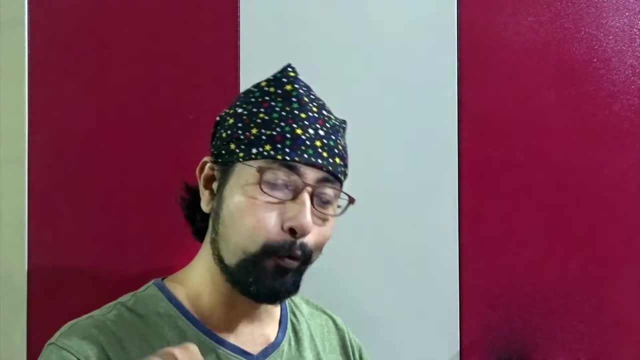 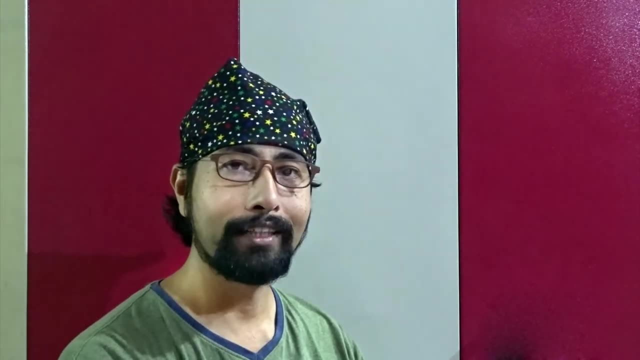 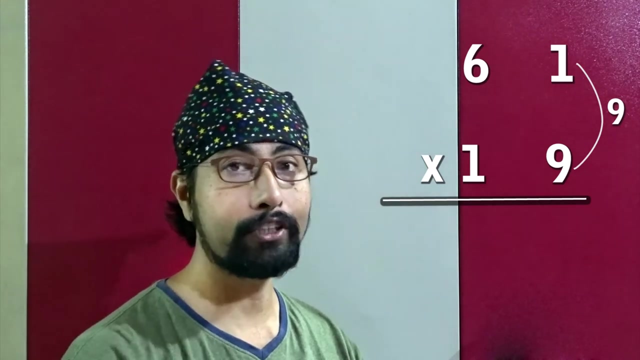 lines, Two lines, But here, only in this video, you will learn this in one line. Yes, it's possible, See this. So 61 into 19.. One, nine, Nine ones are nine. So first of all, nine ones are nine. Now this part we have to do cross. 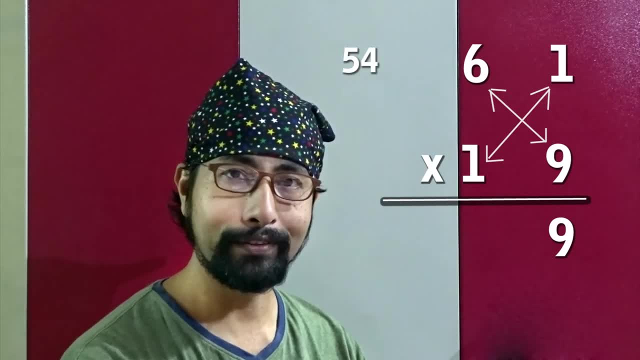 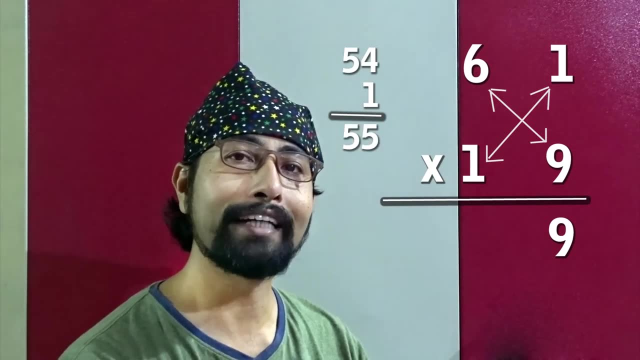 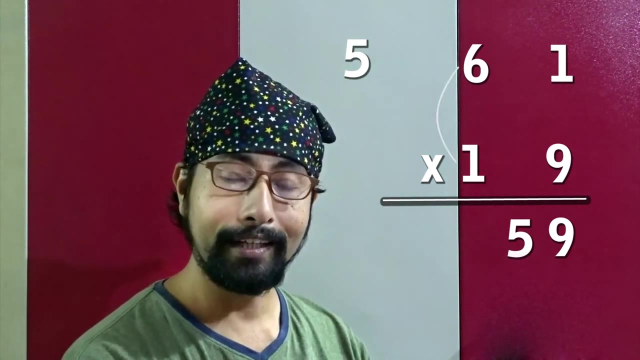 five, Six, nines are 54. Right, And one ones are one, So 54 plus one 55.. So right, only five, And five is in your hand Right Now. six ones are six, And six plus five is equal. 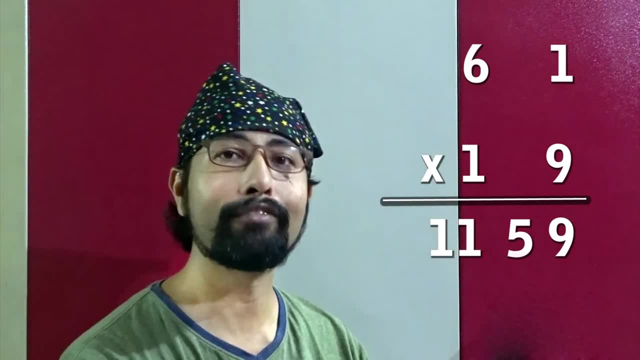 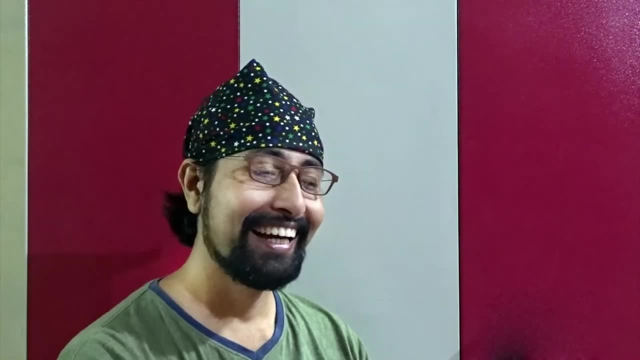 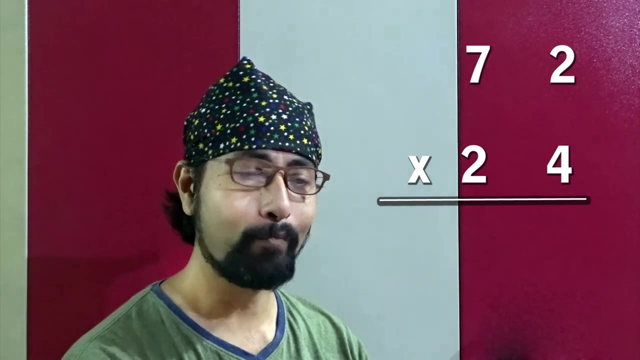 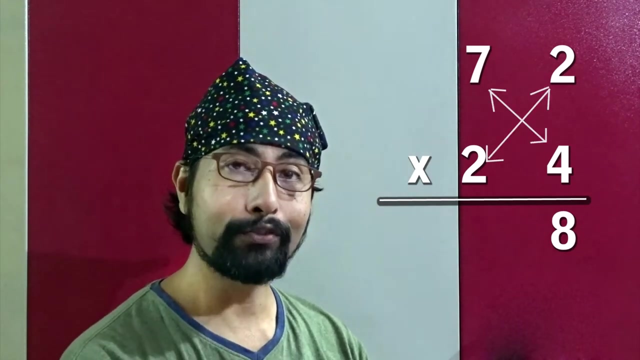 to eleven. So it's eleven hundred fifty-nine In one line. Trust me, You like it. Yes, you like it. Ok, Let's do another one: Seventy-two into twenty-four, Seventy-two into twenty-four. Same way: Four, twos are eight. So fine. Now, cross-wise, Four, sevens are twenty-eight. 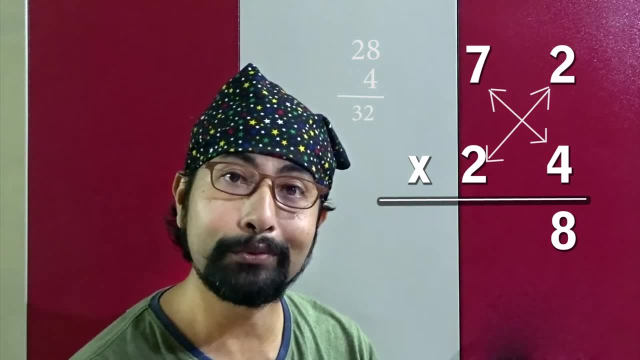 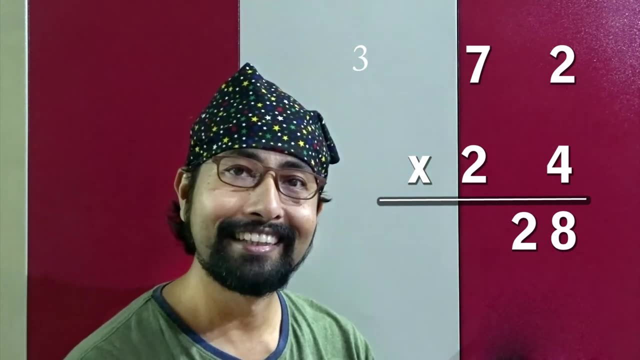 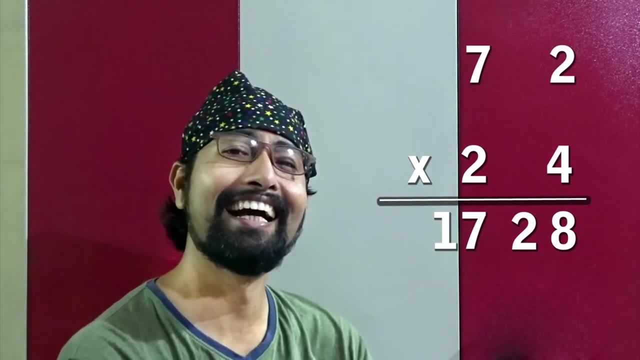 And two. twos are four, Twenty-eight plus four Thirty-two. Just write two, And three is in your hand. Fine, Now the last one: Seven twos are fourteen Plus three, Seventeen, So it's seventeen hundred and twenty-eight. 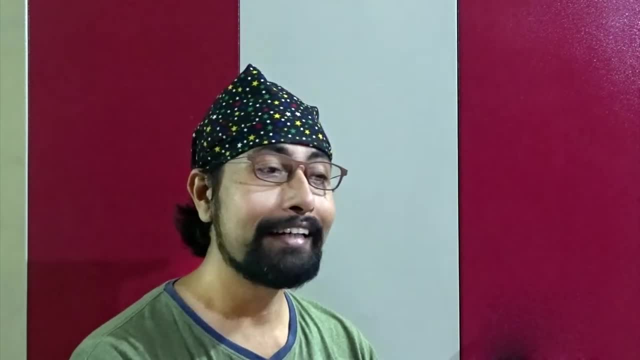 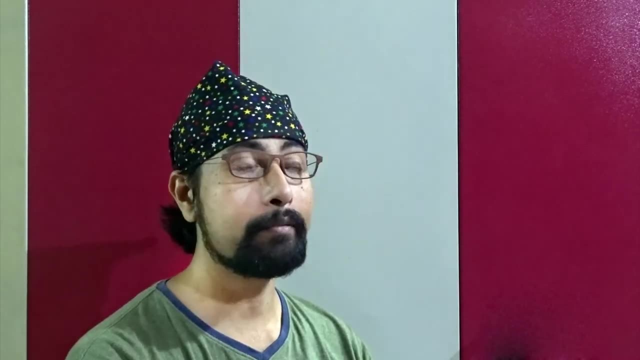 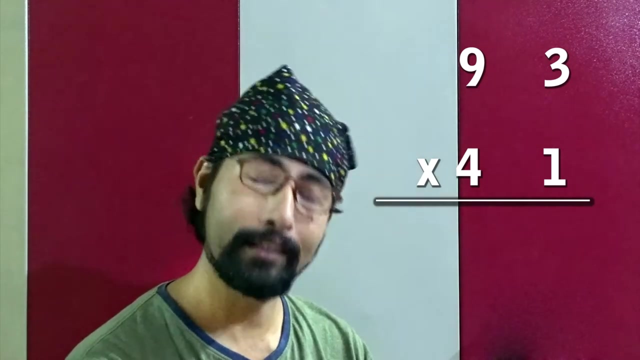 It's mental math. Trust me And do it with me. And next one I'm going to ask you: Yeah, Definitely. I know it's not interactive, but still we can do it. Right. A little bigger number: Write ninety-three into forty-one. It's possible, Try it yourself. Yes, Three. 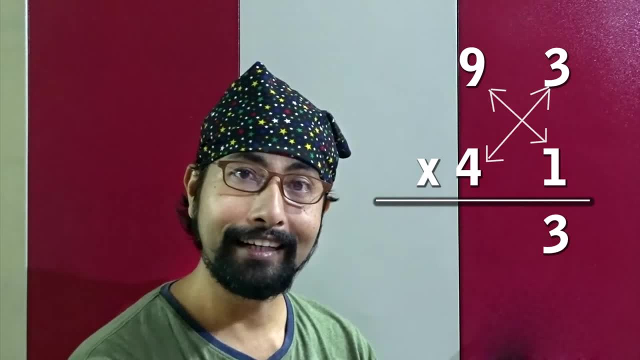 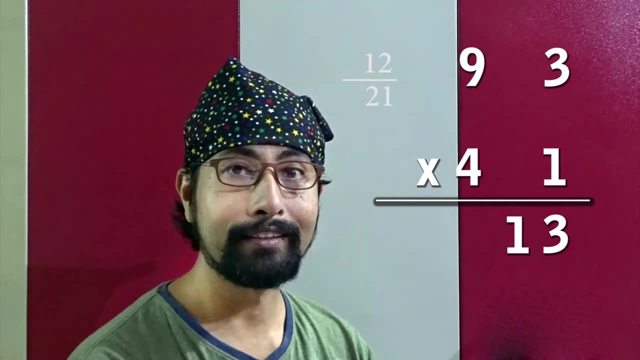 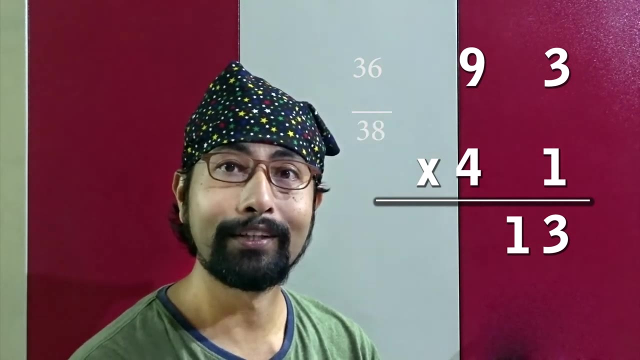 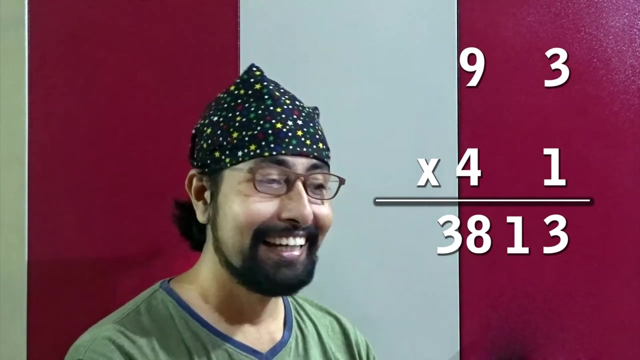 ones are three. Fine, Now nine ones are Nine. Three, fours are Twelve. Twelve plus nine, Twenty-one. Just write one, And two is in your hand. So four nines are Thirty-six Plus two, Thirty-eight, So thirty-eight hundred Thirteen. You like it? See, I'm telling you. 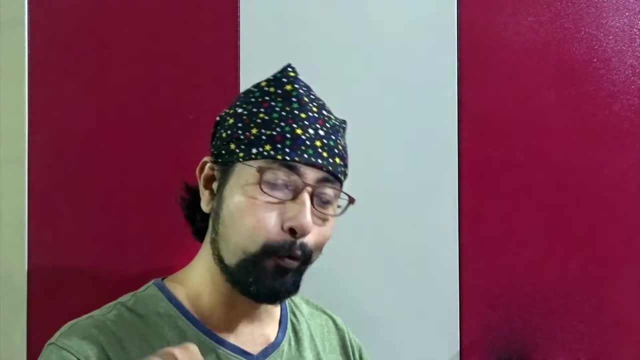 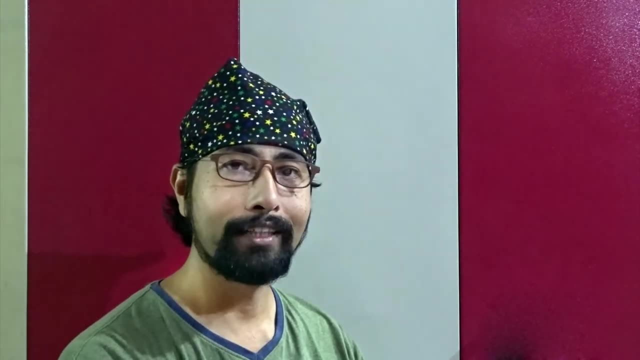 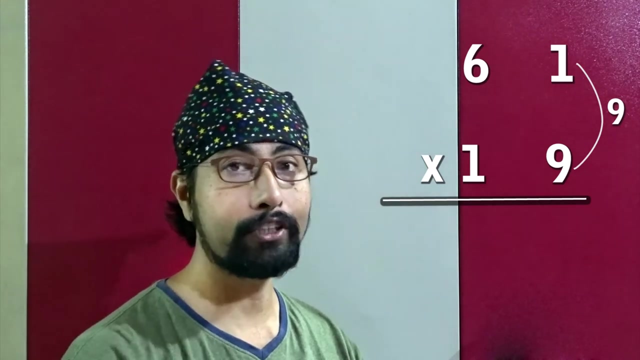 lines, Two lines, But here, only in this video, you will learn this in one line. Yes, it's possible, See this. So 61 into 19.. One, nine, Nine ones are nine. So first of all, nine ones are nine. Now this part we have to do cross. 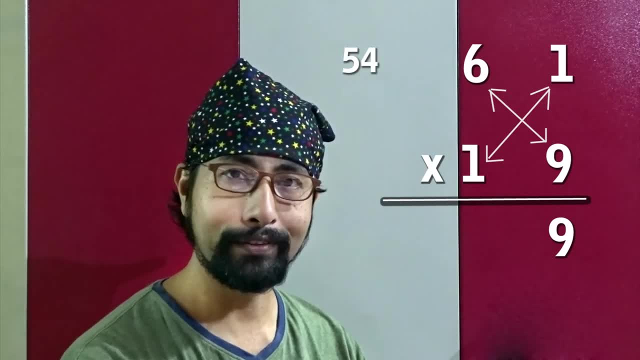 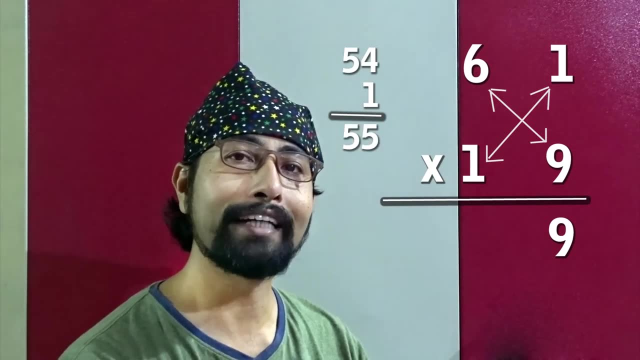 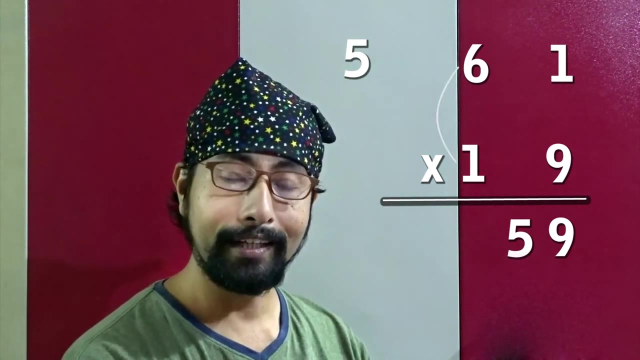 fives, Six, nines are 54. Right, And one ones are one, So 54 plus one 55.. So right, only five, And five is in your hand Right Now. six ones are six, And six plus five is equal. 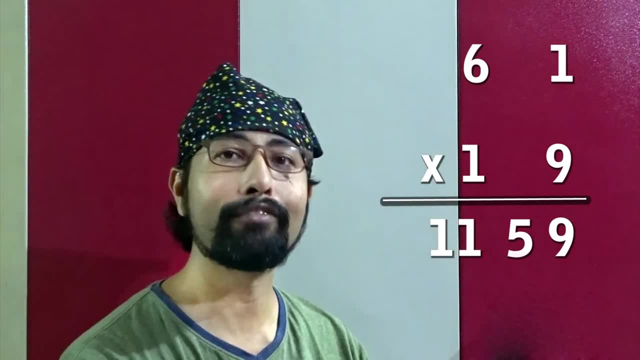 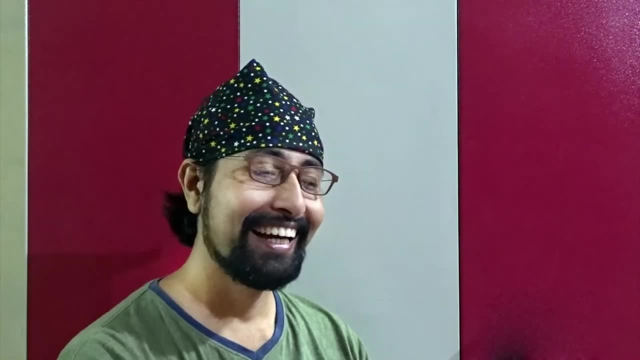 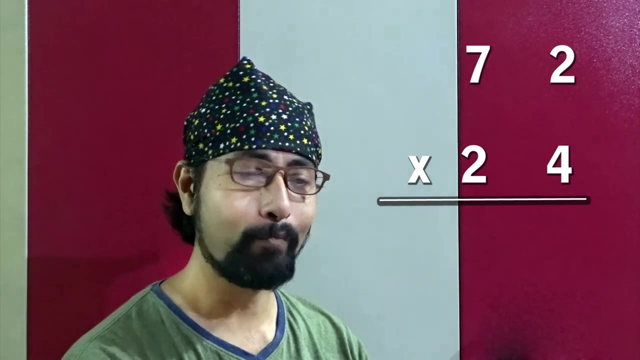 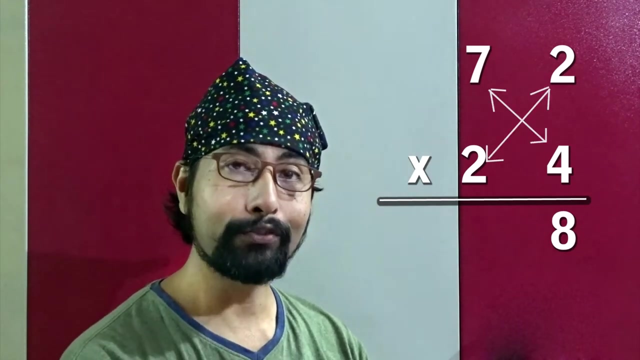 to eleven. So it's eleven hundred fifty-nine In one line. Trust me, You like it. Yes, you like it. Ok, Let's do another one. Seventy-two into twenty-four, Seventy-two into twenty-four. Same way: Four, twos are eight. So fine, Now cross fives. Four, sevens are twenty-eight. 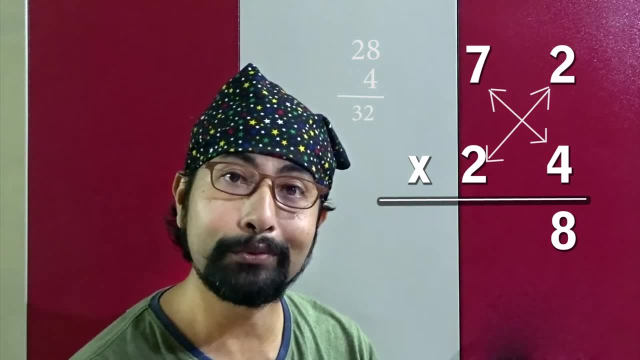 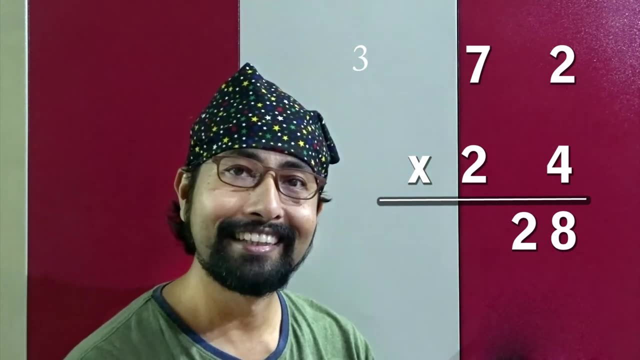 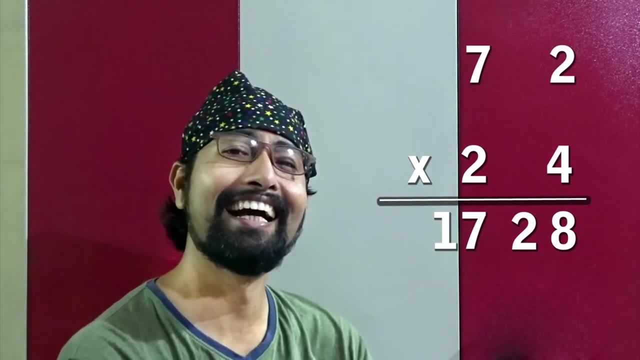 And two. twos are four, Twenty-eight plus four Thirty-two. Just write two, And three is in your hand. Fine, Now the last one: Seven twos are fourteen Plus three, Seventeen, So it's seventeen hundred and twenty-eight. 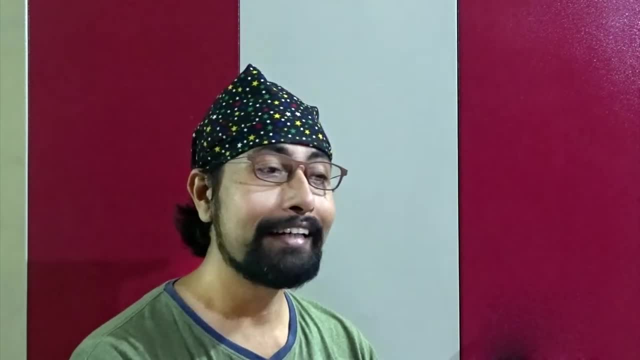 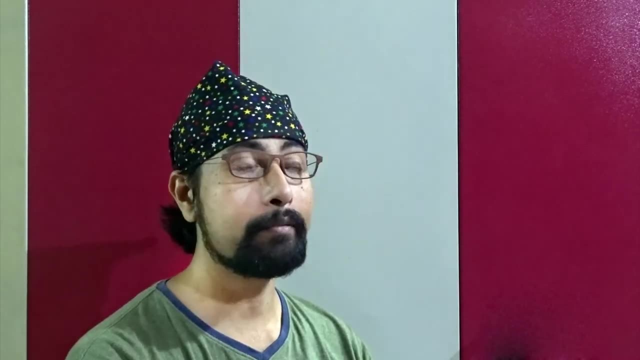 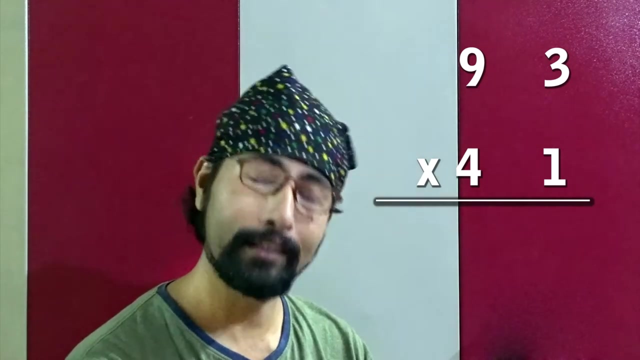 It's mental math. Trust me And do it with me. And next one I'm going to ask you: Yeah, Definitely. I know it's not interactive, but still we can do it. Right. A little bigger number: Write ninety-three into forty-one. It's possible, Try it yourself. Yes, Three. 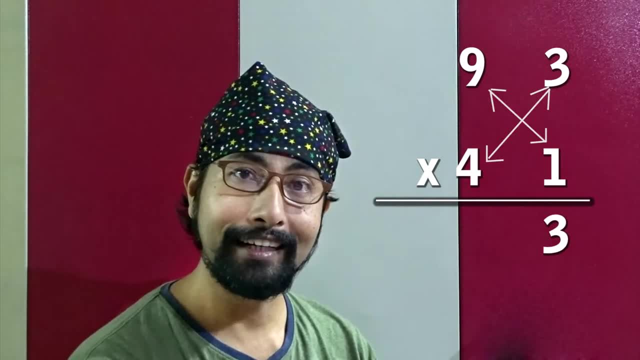 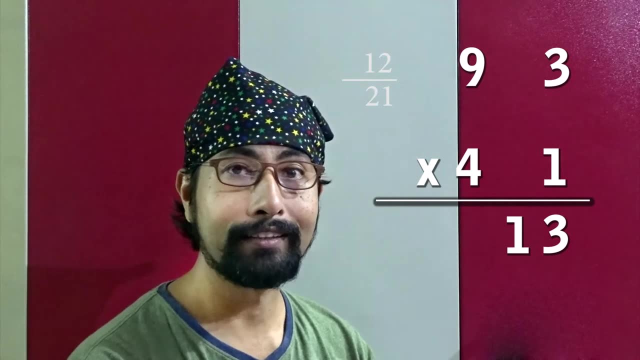 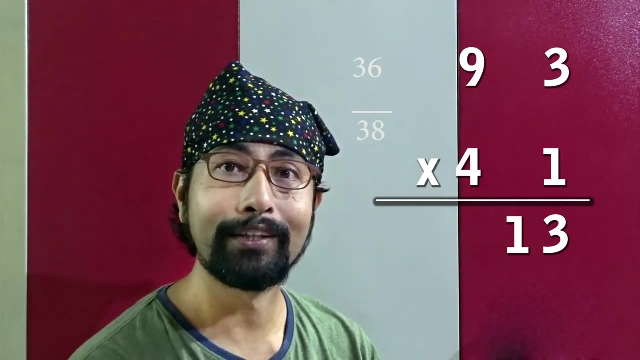 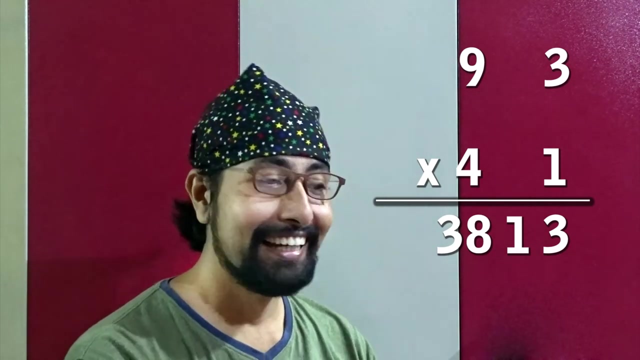 ones are three. Fine, Now nine ones are nine. Three, fours are twelve, Twelve plus nine, Twenty-one. Just write one, And two is in your hand. So four nines are thirty-six Plus two, Thirty-eight, So thirty-eight hundred Thirteen. You like it? See, I'm telling you, This is the only. 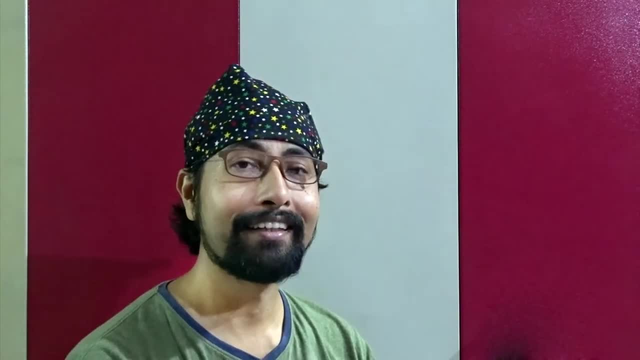 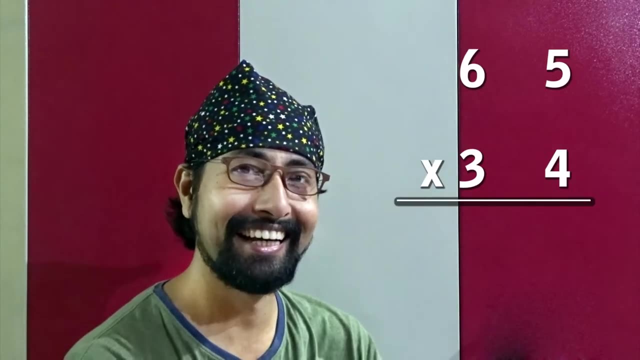 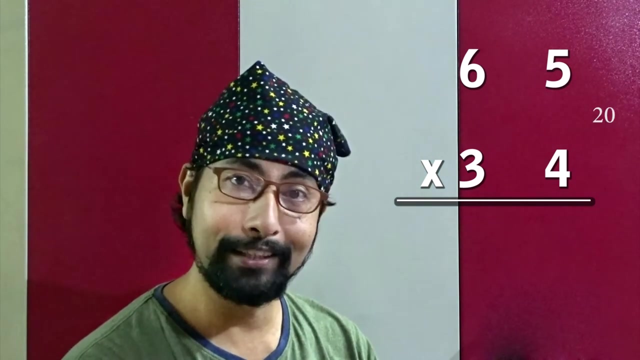 This is the only channel where you will find this in one line, Next one like sixty-five into thirty-four. Little bit complex, Little bit complex. Calculate more in your mind. So five fours are Twenty. Zero is there. Two is in your hand, Six fours. 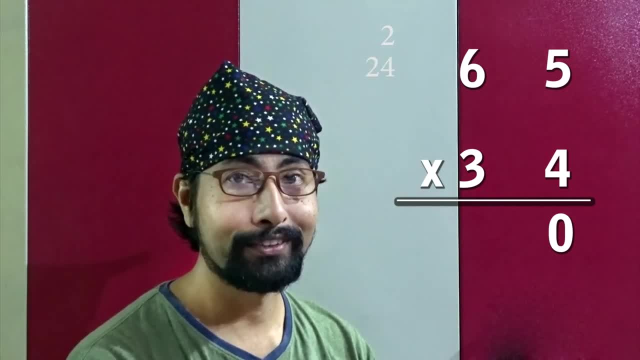 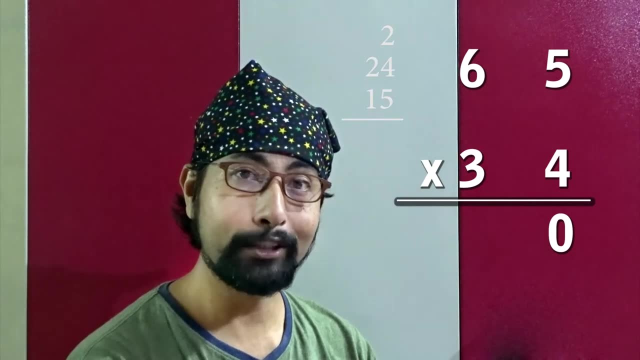 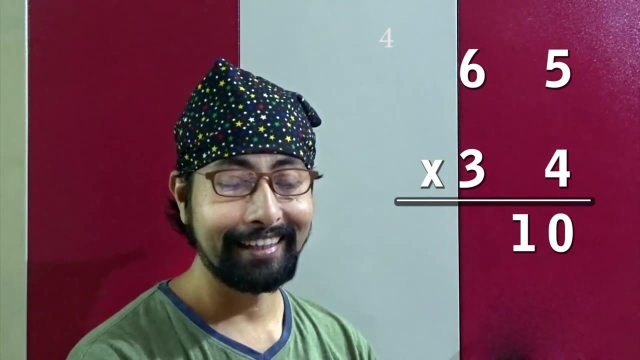 are Twenty-four. Three fives are Fifteen. Fifteen plus twenty-four, Thirty-nine, Thirty-nine plus two, Forty-one, So one is there. Now you have four in your hand, So last one: Six. threes are Eighteen. 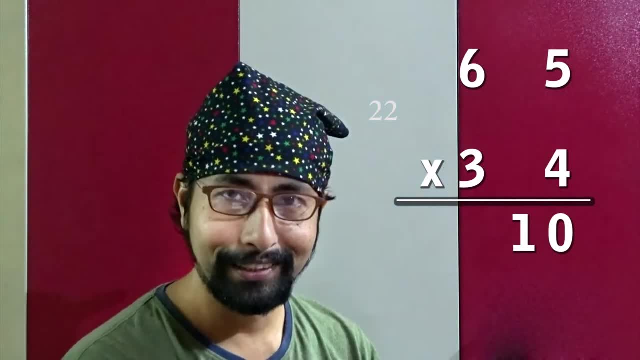 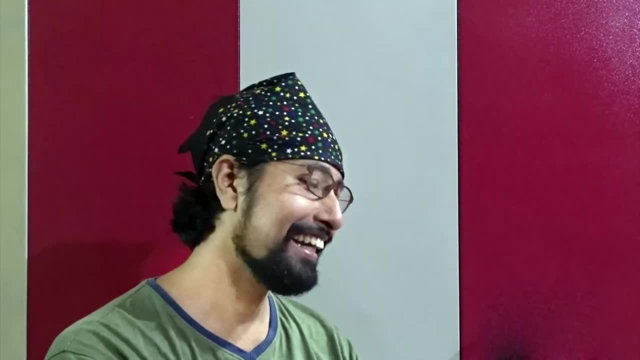 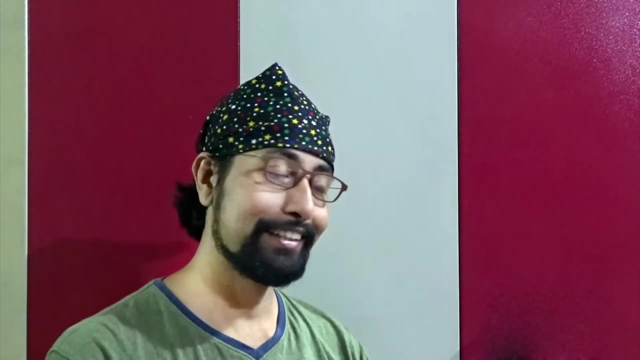 Last four, Twenty-two, So it's twenty-two hundred and ten. You like it? So next one, I'm not going to leave you, Trust me. Do it with me, Please, Please For yourself, Do it for you, Do it for me. 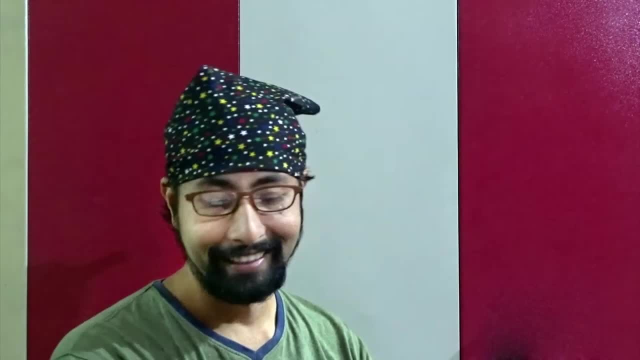 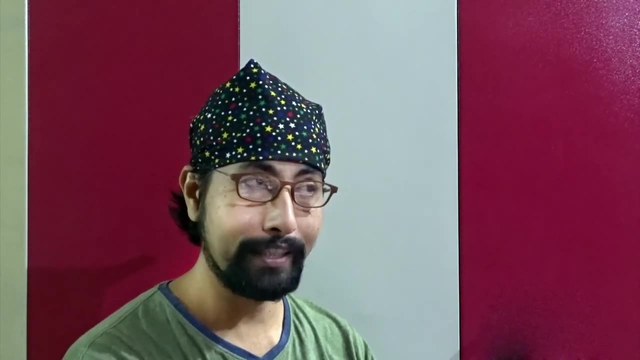 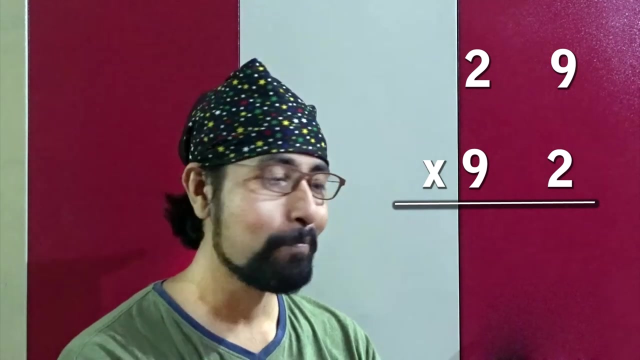 Do it for yourself, It's for your brain, basically. So last one, we can try with an easy number like twenty-nine into ninety-two, Twenty-nine into twenty-two, Possible. So another process: Nine twos are Eighteen. Eight is there? Now one is in your hand. 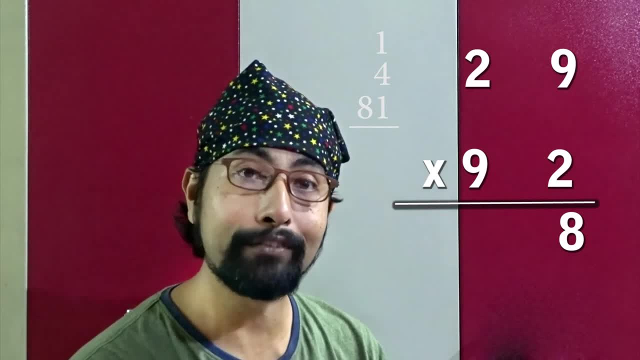 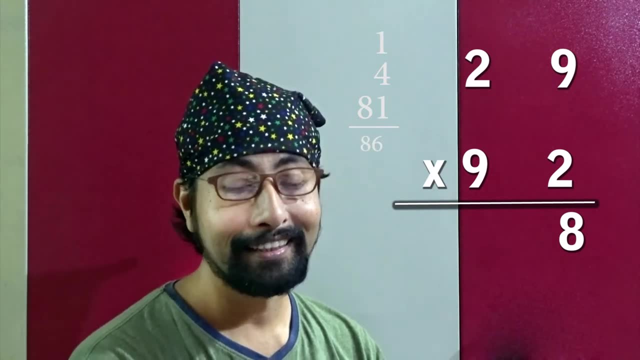 Two, twos are four, Nine, nines are Eighty-one. Eighty-one plus four, Eighty-five. Well done, Great work, Bye, bye. one is your hand, so 86, six. just write six. now eight is in your hand, now nine. 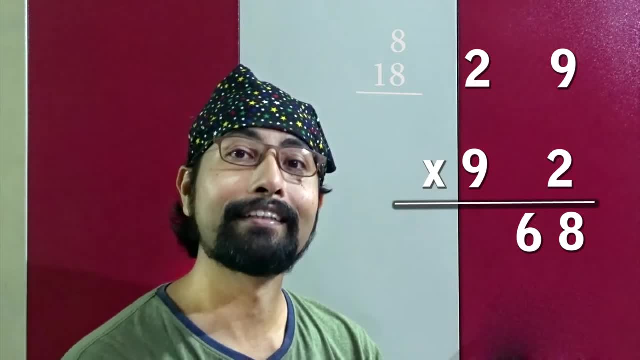 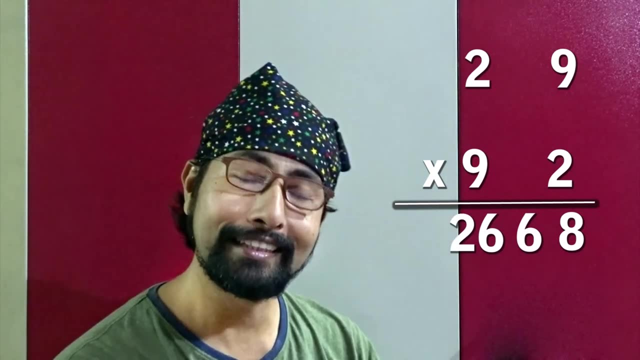 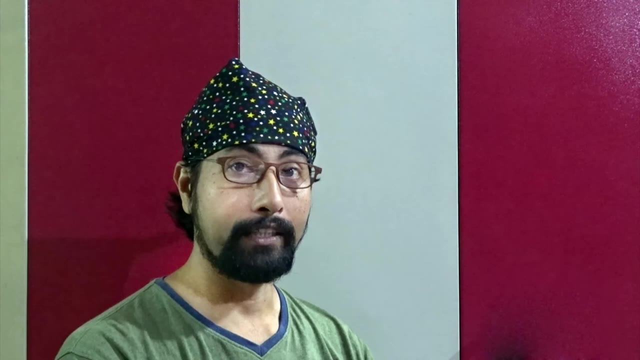 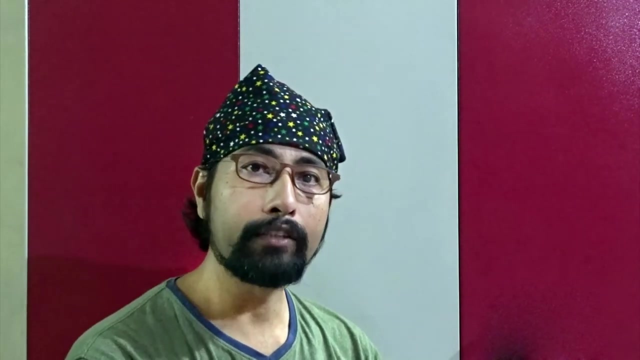 twos are 18, 18 plus 8, 26. so the final answer is 26 and red and 68. you like it, you must like it and, trust me, you just practice like this and you can do it even for a bigger number. it's a matter of practice. if you practice, more you. 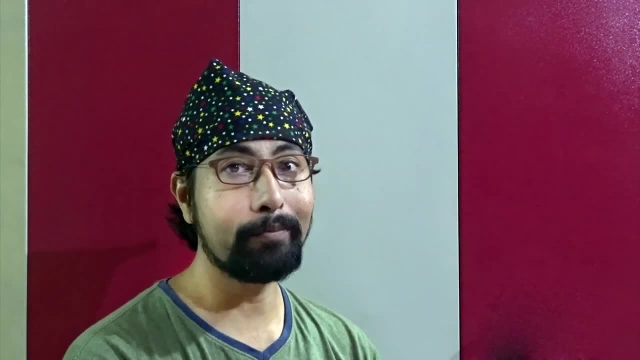 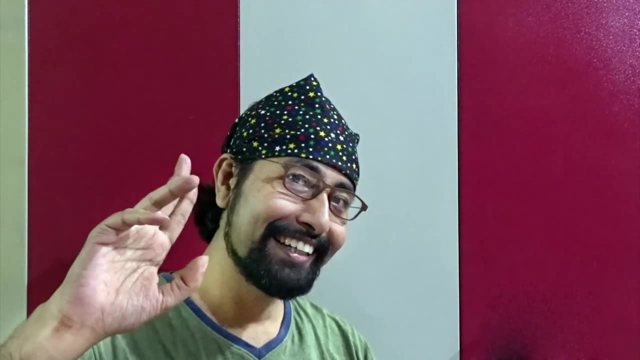 will feel comfortable with maths, and this way we can develop our brain easily, just like this. so that's it for today. bye, bye. 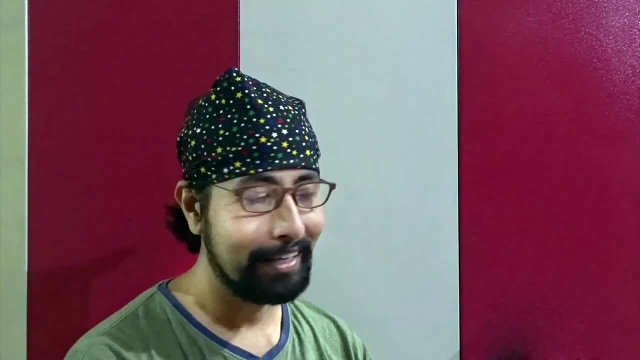 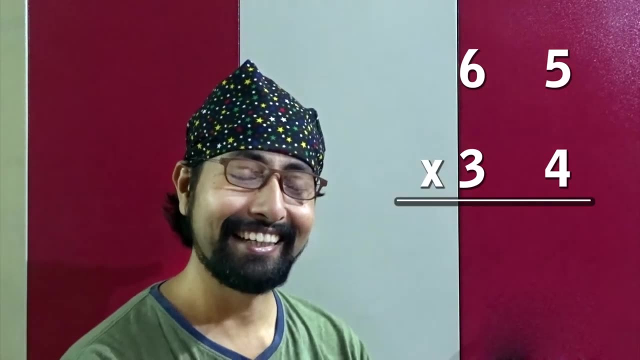 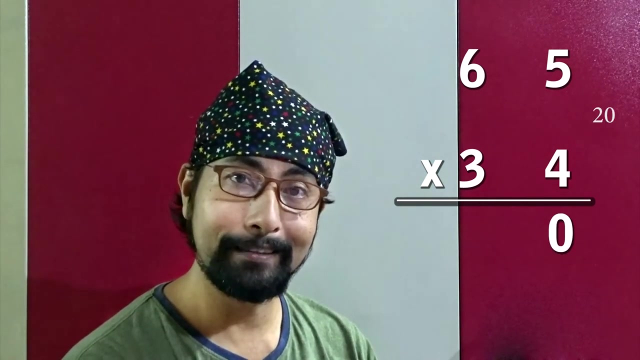 channel where you will find this in one line, Next one Like sixty-five into thirty-four. Little bit complex, Little bit complex. Calculate more in your mind. So five, fours are twenty. Zero is there. Two is in your hand, Six, fours. 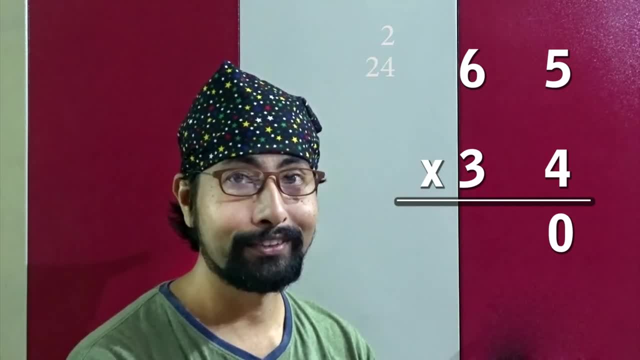 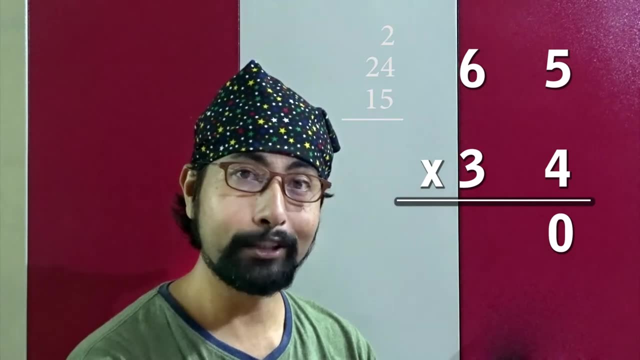 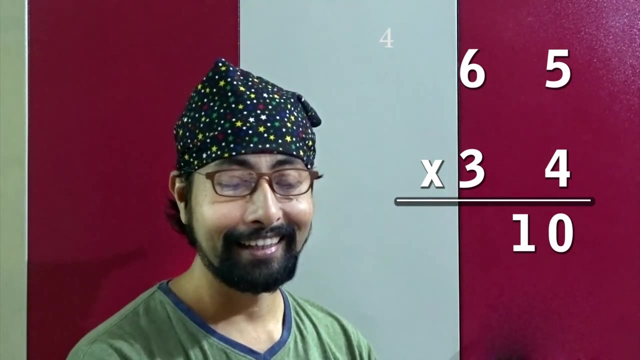 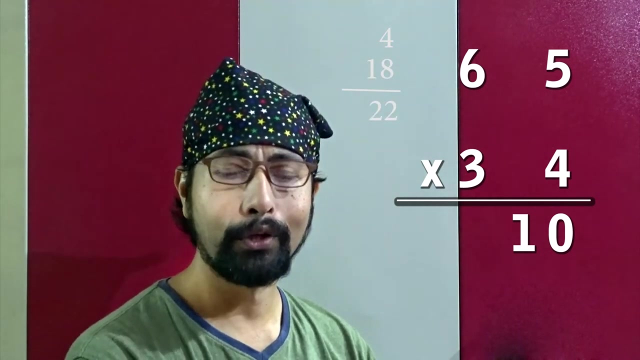 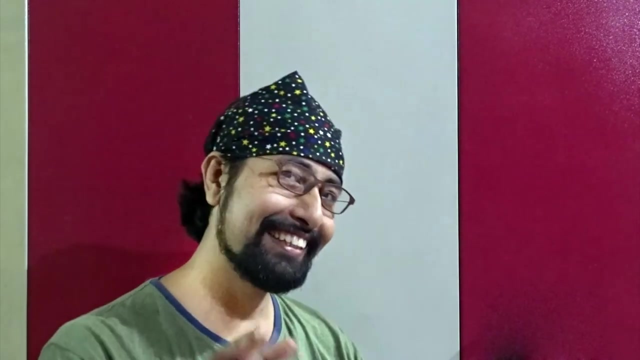 are twenty-four. Three fives are fifteen. Fifteen plus twenty-four, Thirty-nine, Thirty-nine plus two, Forty-one, So one is there Now. you have four in your hand, So last one. Six, threes are eighteen. Last four: Twenty-two, So it's twenty-two hundred and ten, You like it? So next one. 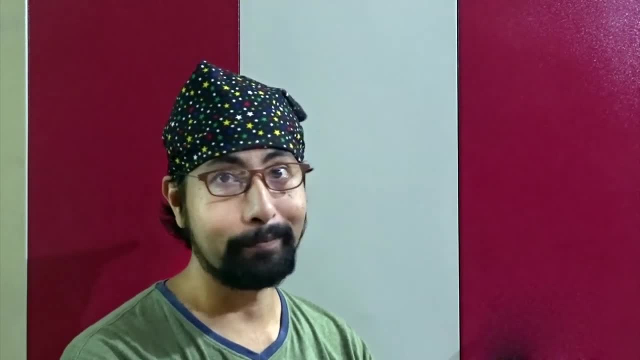 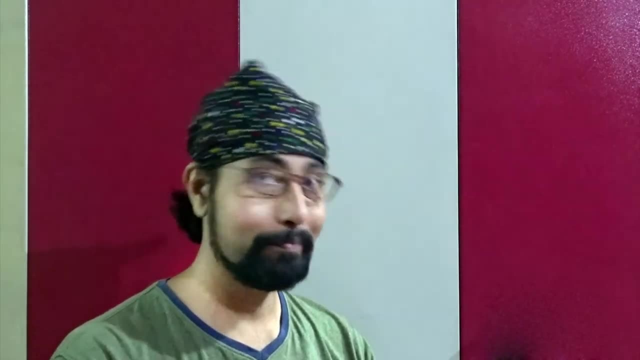 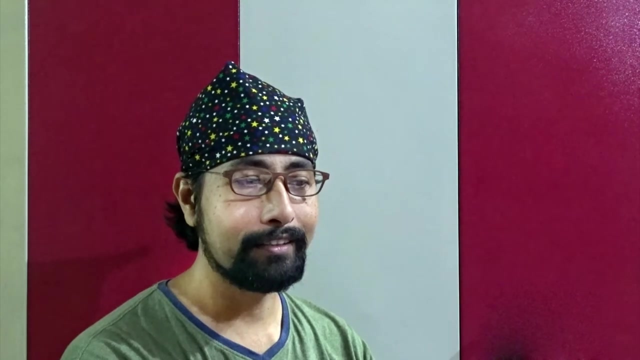 I'm not going to leave you, Trust me. Do it with me, Please, Please For yourself, Do it for you, Do it for me. It's for your brain, basically. So last one, we can try with an easy number Like twenty-nine. 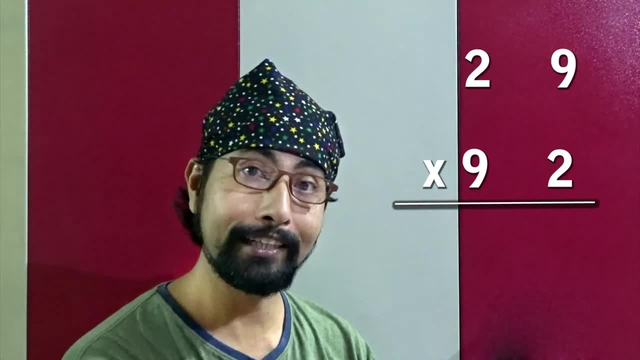 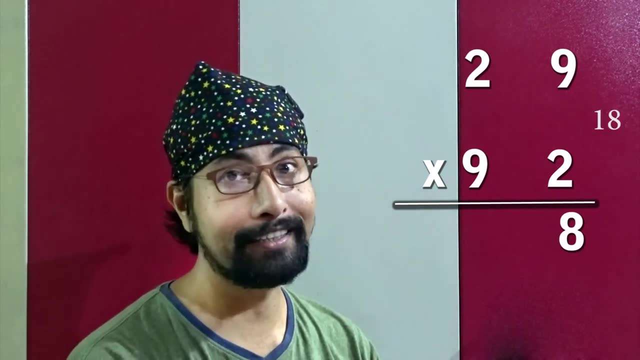 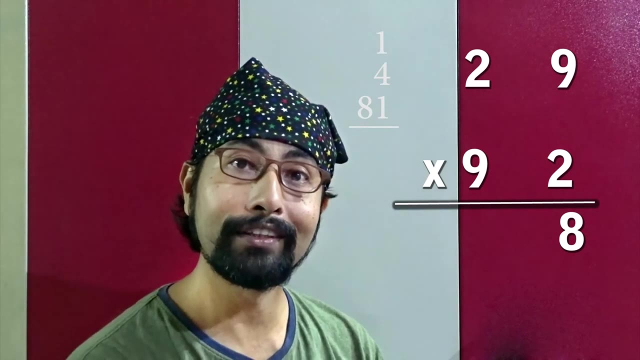 into ninety-two, Twenty-nine into twenty-two, Possible. So know the process. Nine twos are Eighteen. Eight is there, Not one is in your hand. Two twos are four. Nine nines are Eighty-one. Eighty-one plus four, Eighty-five. 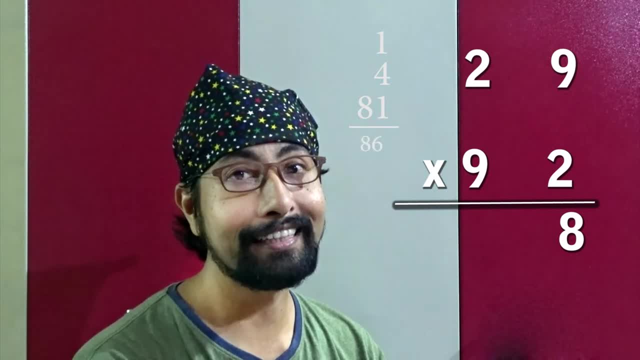 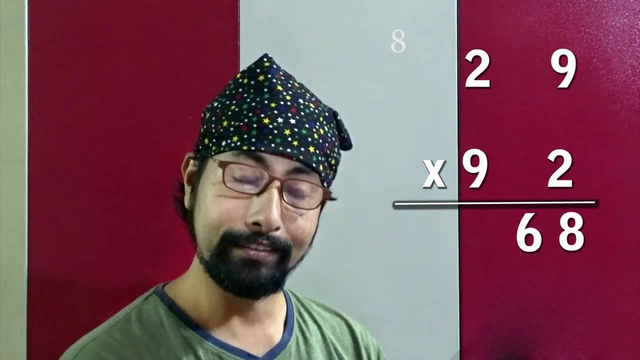 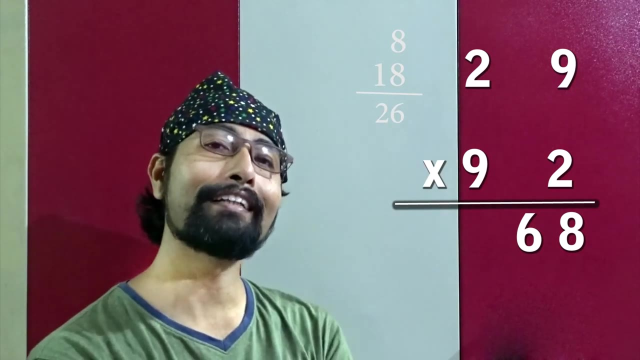 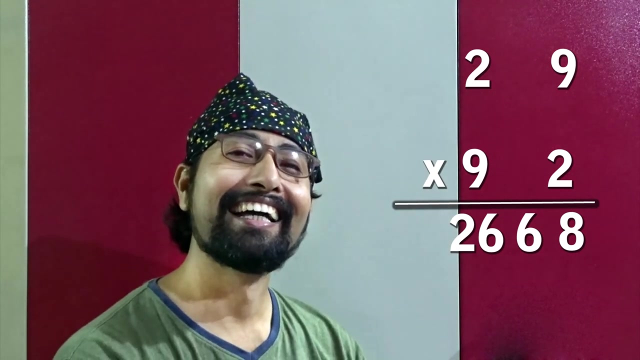 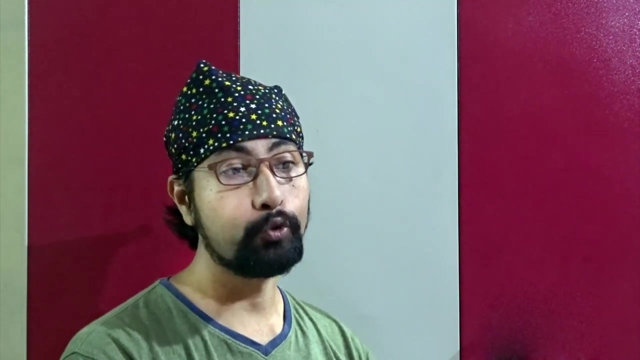 one is your hand. so 86, 6, just write 6. now 8 is in your hand. now 9 to the 18, 18 plus 8, 26, so the final answer is 26 and 68. you like it, you must like it and trust me, you just practice like this and you can do it, even. 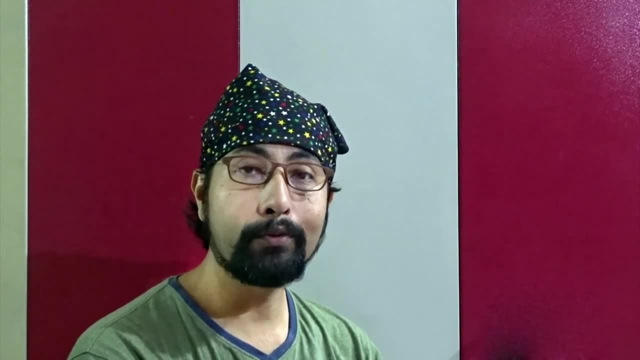 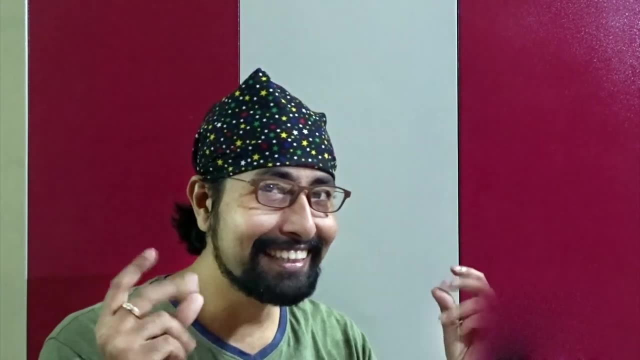 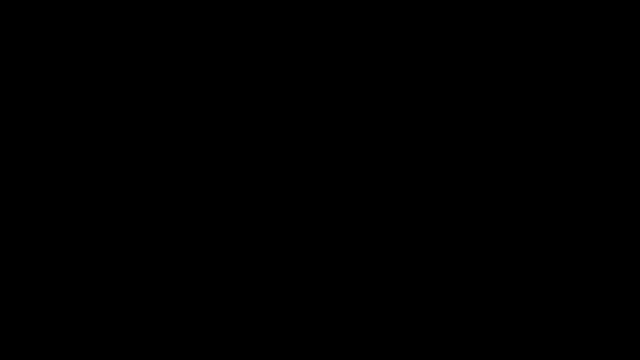 for a bigger number. it's a matter of practice. if you practice more, you will feel comfortable with maths, and this way we can develop our brain easily, just like this. so that's it for today. bye you.